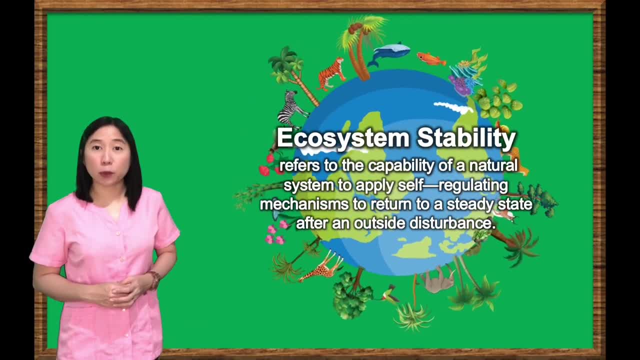 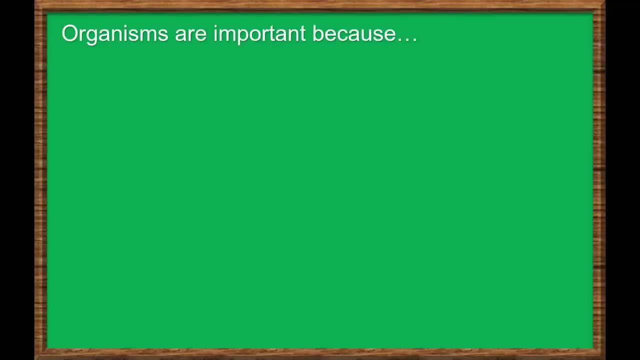 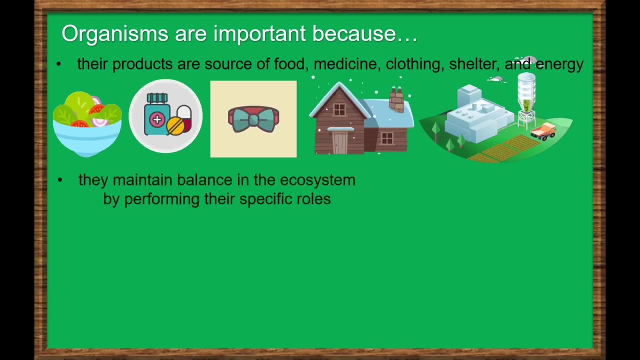 The stability of an ecosystem can be described as the resilience to withstand changes that may occur in the environment. Organisms are important because their products are source of food, medicine, clothing, shelter and energy. They maintain balance in the ecosystem by performing their specific roles. 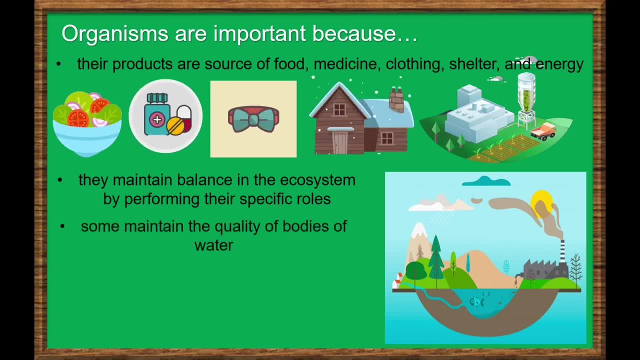 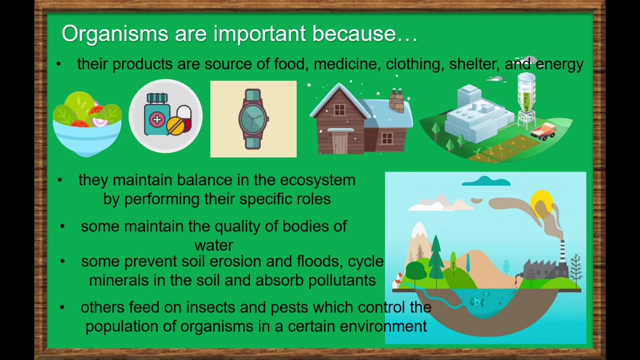 Some maintain the quality of bodies of water, Some prevent soil erosion and floods, cycle minerals in the soil and absorb pollutants, And others feed on insects and pests which control the population of organisms in a certain environment. Thus, organisms maintain a balanced and stable ecosystem. 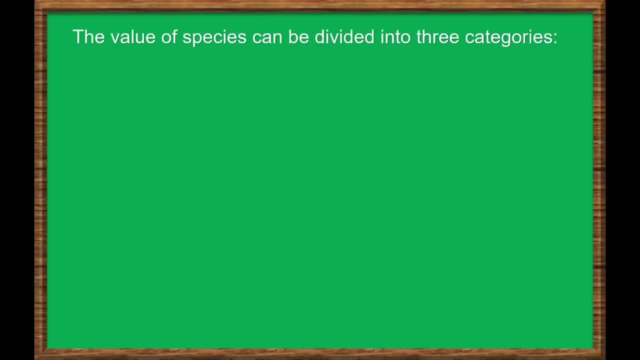 Lesson 11. Organisms and their ecosystem- Lesson 12. Organisms and their ecosystem- Lesson 13. Organisms and their ecosystem- Lesson 14. Organisms and their ecosystem- Lesson 15. Organisms and their ecosystem In general, the value of species or organisms can be divided into three categories. 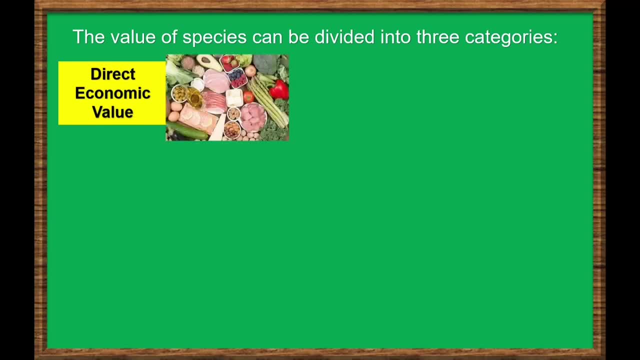 We have direct economic value, which means a species is considered to have direct economic value if their products are source of food, medicine, clothing, shelter and energy. For example, some medicines being used nowadays have formulation extracted from plants or animals. Next is indirect economic value. 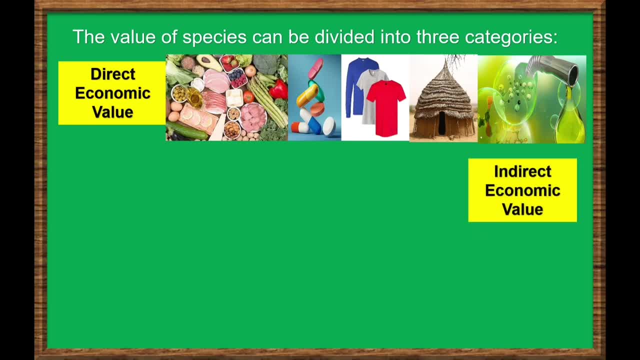 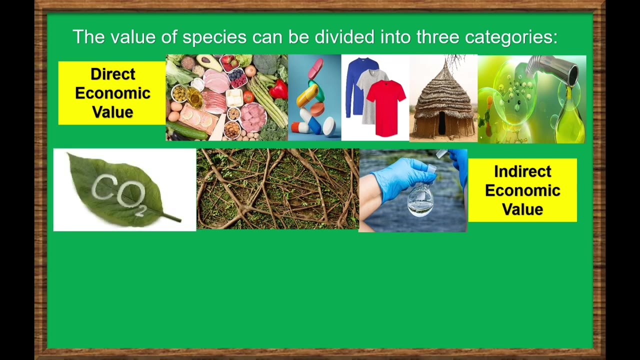 A species has indirect economic value if there are benefits: benefits produced by the organisms without using them. for example, certain species maintain the chemical quality of natural bodies of water, prevent soil erosion and floods, cycle materials in the soil and absorb pollutants. and, lastly, aesthetic value. a lot of species provides. 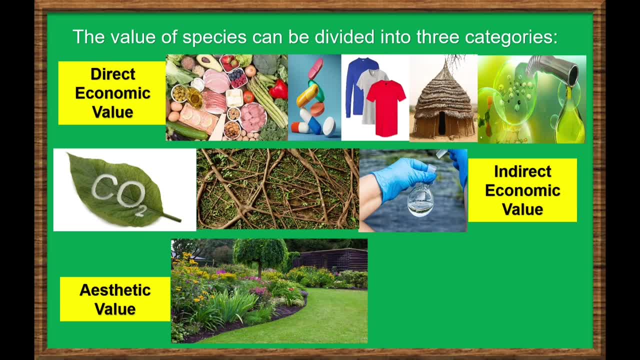 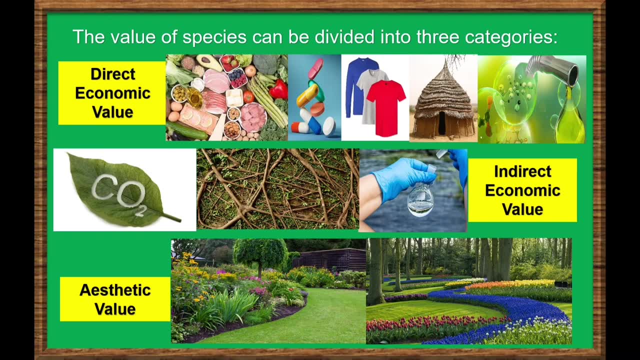 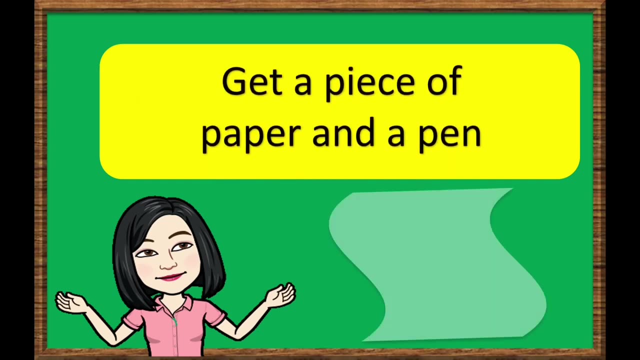 visual or artistic enjoyment, like a forested landscape and the calming beauty of a natural park, or they may be used for spiritual meditation, like the prayer mountains. let us perform a simple activity: get a piece of paper and a pen. number your paper from 1 to 10.. let's start. 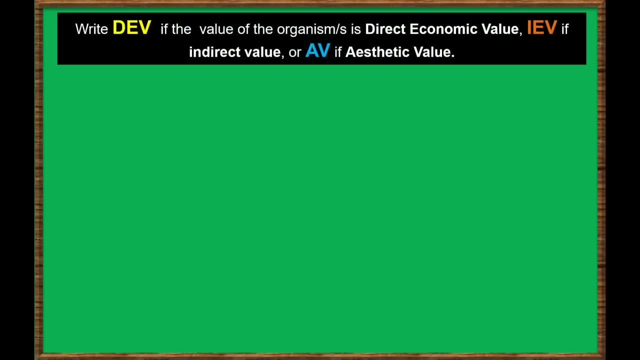 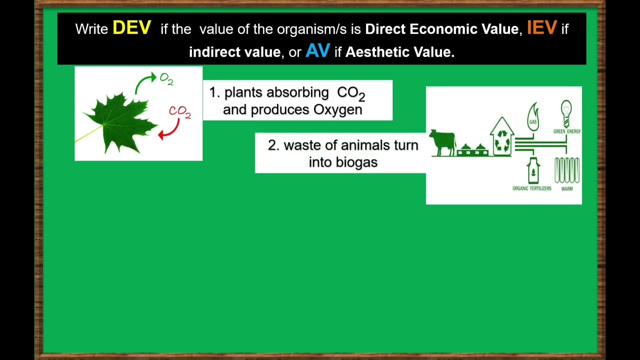 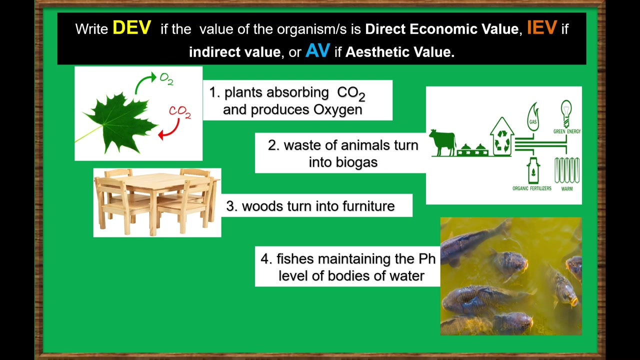 write dev if the value of the organisms has direct economic value, IEV if indirect value or AV if aesthetic value. let's start. number one: plants absorbing carbon dioxide and produces oxygen. number two: ways of animals turn into biogas. number three: Woods turn into furniture. number four: fish are fishes maintaining the pH level of bodies of water. 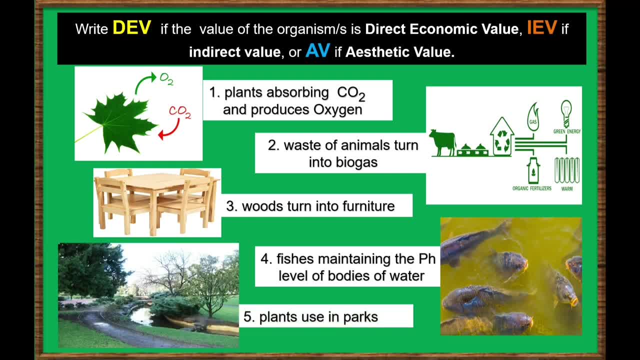 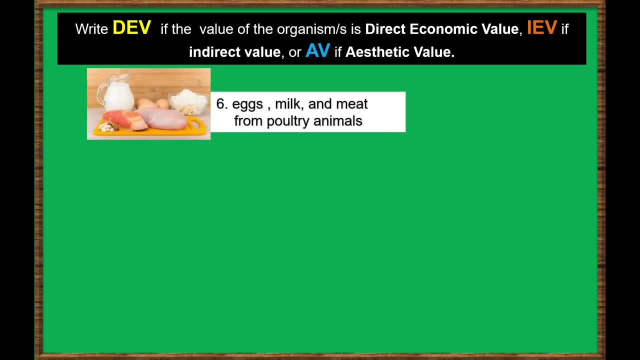 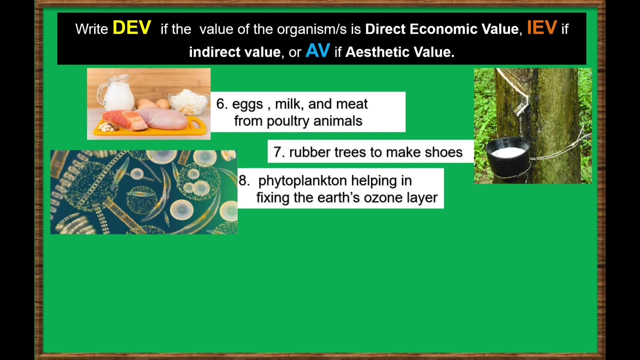 Plants used in parks. Number six: eggs, milk and meat from poultry animals. Number seven: rubber trees to make shoes. Number eight: phytoplankton helping in fixing the earth's ozone layer. Number nine: carabao helping farmers in plowing the fields. 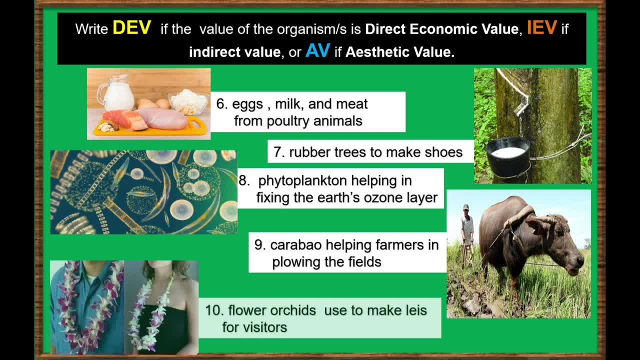 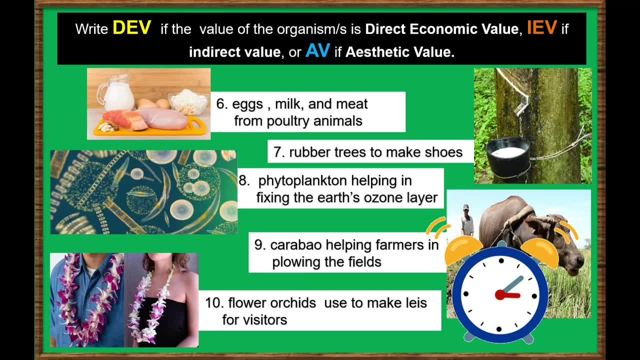 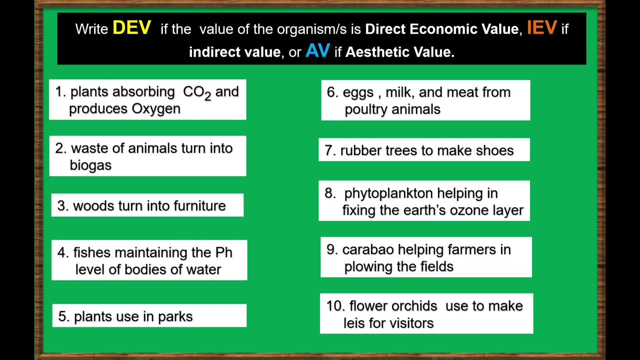 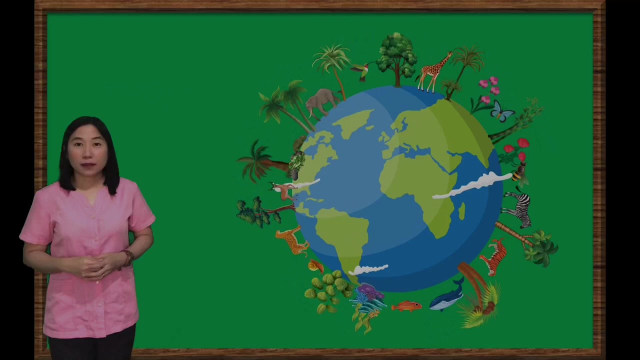 And number ten: flower orchids used to make lace for visitors. Let's see how you did well in our activity. Let's check Number two, Number three, Number four and five, Number six and seven, Number eight and nine: number two, Since you now know the importance of biodiversity. 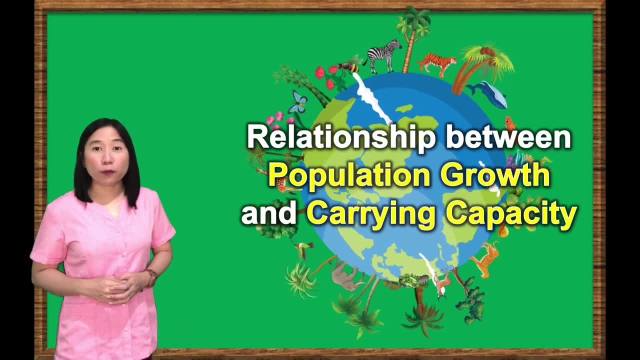 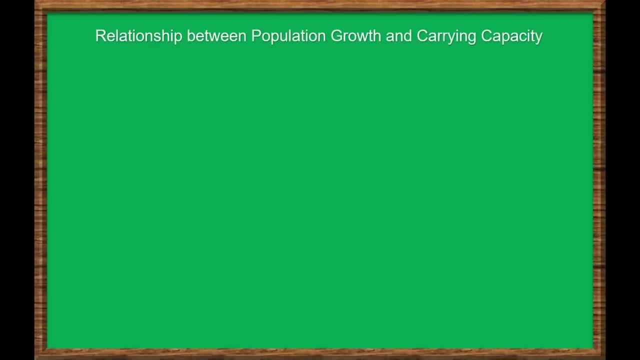 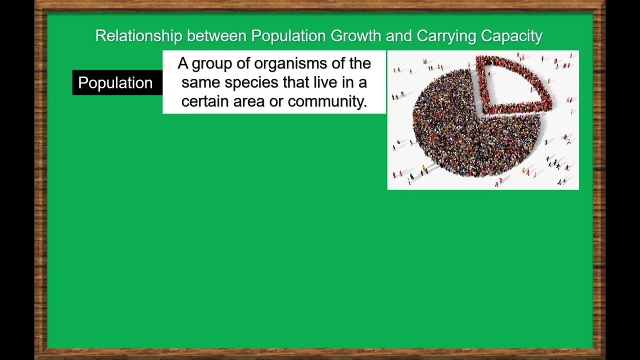 let us learn how the population of organisms in an ecosystem affect biodiversity. Relationship between population growth and carrying capacity. Population is a group of organisms of the same species that live in a certain area or community. Scientists regularly monitor the number of populations of organisms in an area. 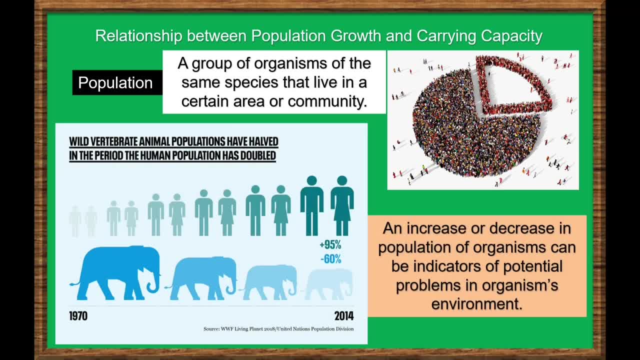 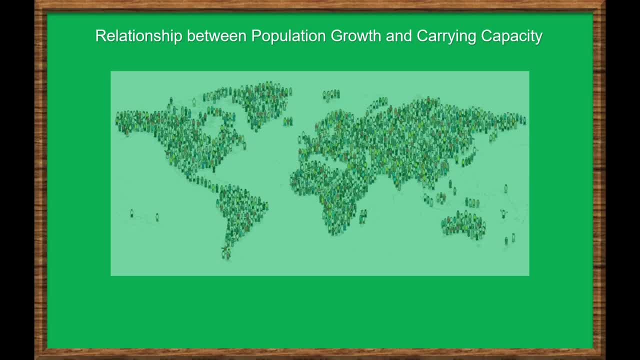 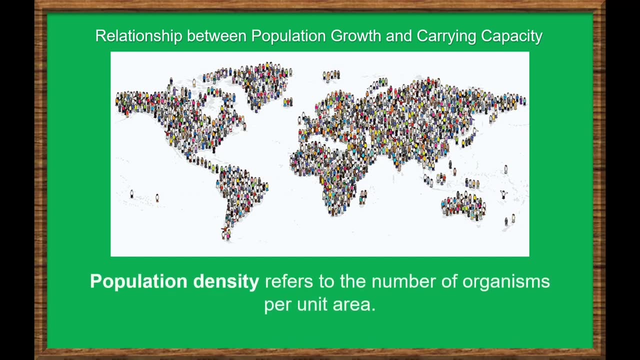 because an increase or decrease in population can be indicators of potential problems in organisms' environment. As a population grows in an area, a population may experience the effects of increased densities. Population density refers to the number of organisms. Population density refers to the number of organisms per unit area. 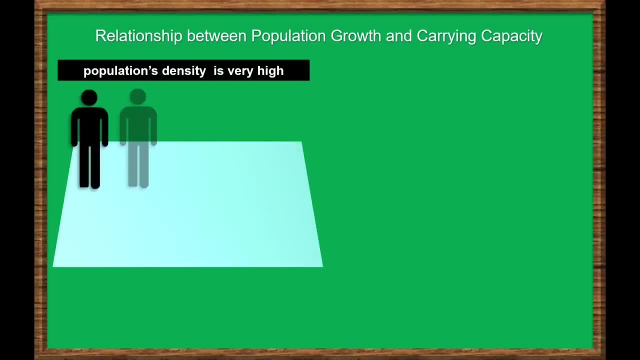 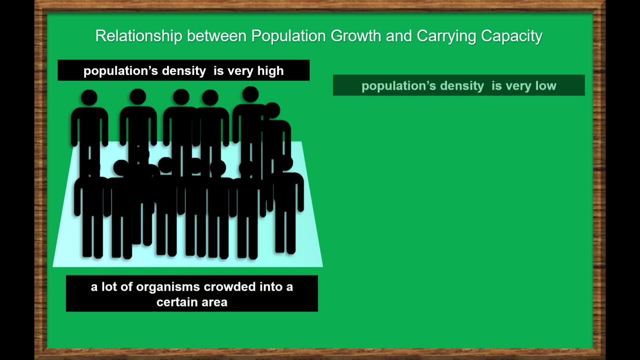 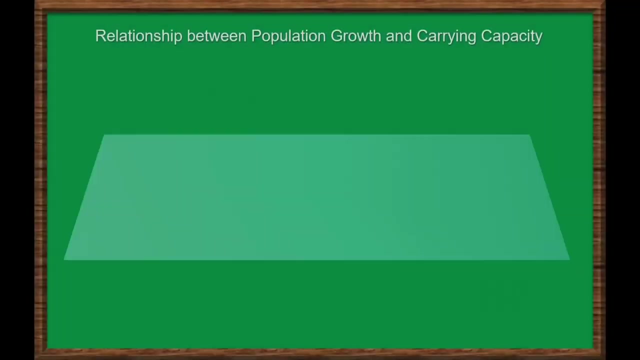 Please take note that if the population's density is very high, it means that there are a lot of organisms crowded into a certain area, But if the population's density is very low, this means that there are few organisms in an area. As a population grows in an area, a population may experience the effects of increased densities. 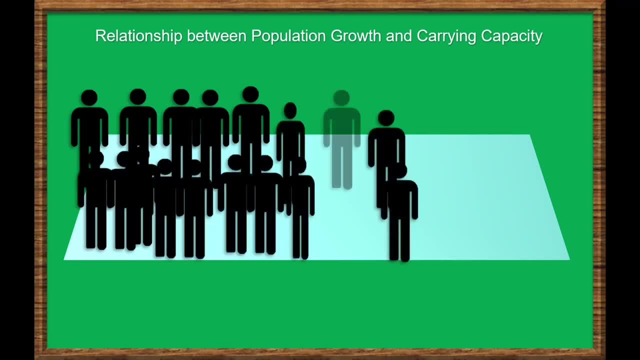 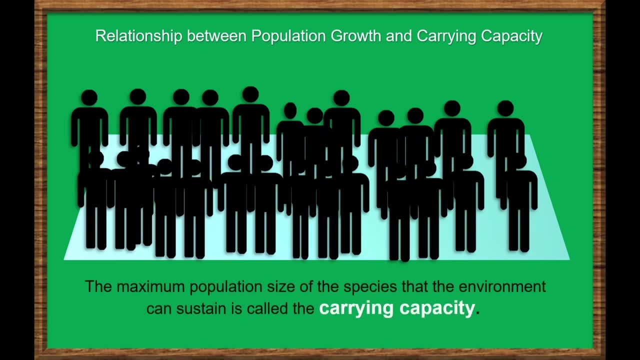 In a given area. a population may experience the effects of increased densities. In a given area, the maximum population size of the species that the environment can sustain is called the carrying capacity. Carrying capacity is determined by the amount of available resources like food, water or habitat. 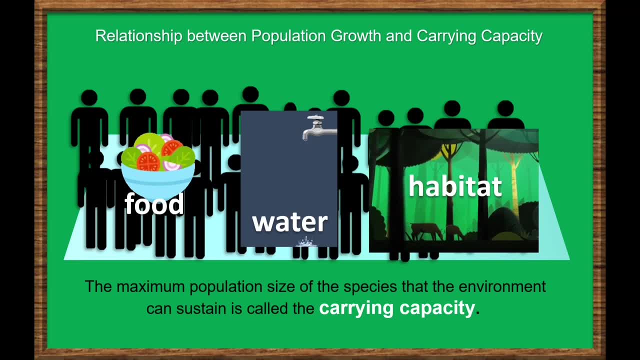 If the population grows indefinitely, competition will increase between organisms and less and less resources will be available to sustain the population. that can lead to density dependence. For this reason, it may cause an ecosystem to collapse. to collapse, remember. a growth of population can be limited by two main 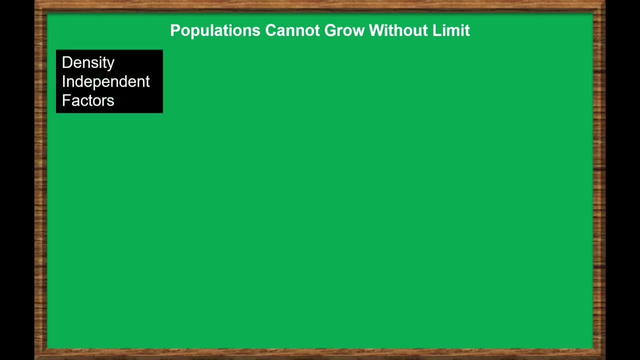 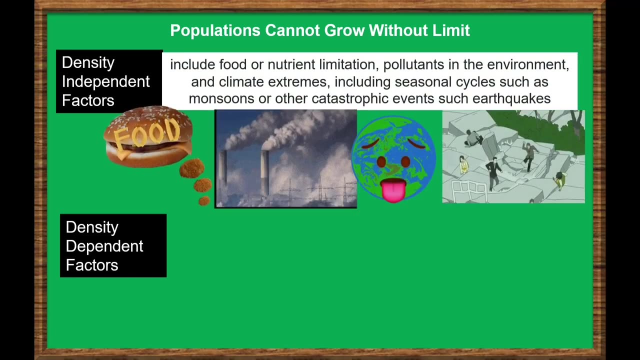 factors, density independent factors and density dependent factors. in density independent factors, a growth of population may be limited by the following: food or nutrient limitation, pollutants in the environment and climate, extremes, including seasonal cycle such as monsoon, or other catastrophic events such as earthquakes, while in density dependent factors. 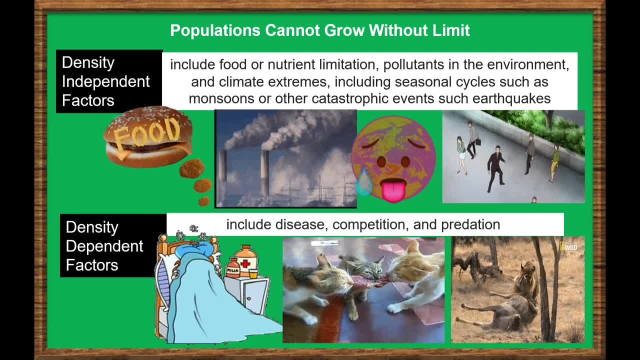 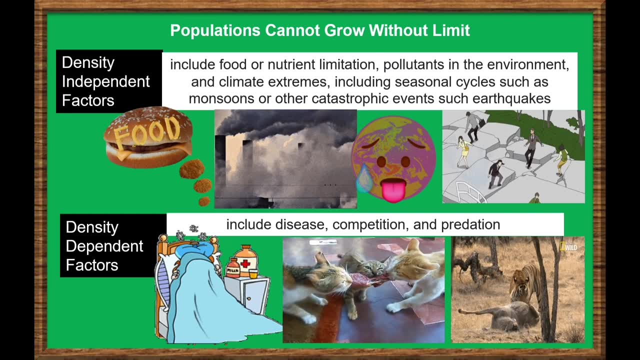 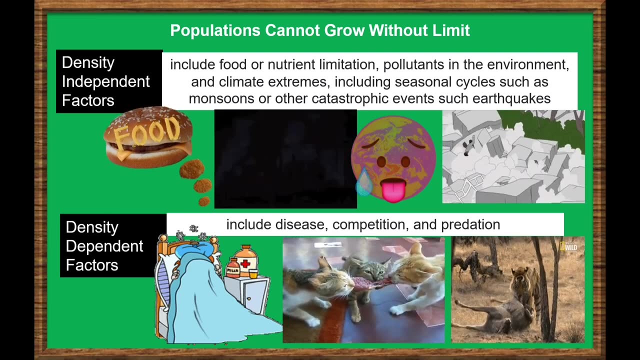 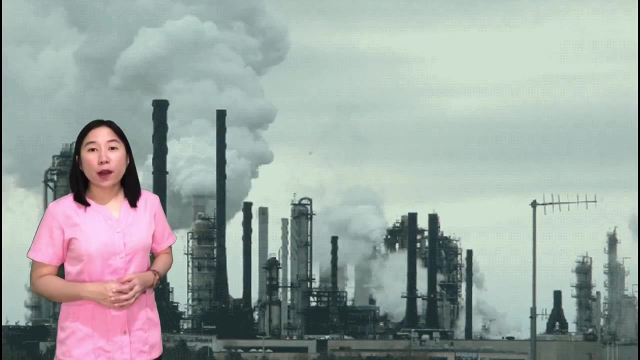 population can be limited by diseases, competition and predation. density dependent factors can have either a positive or a negative correlation to population size. with a positive relationship, this limiting factors increase with the size of the population and limit growth as population size increases the stability of our environment.